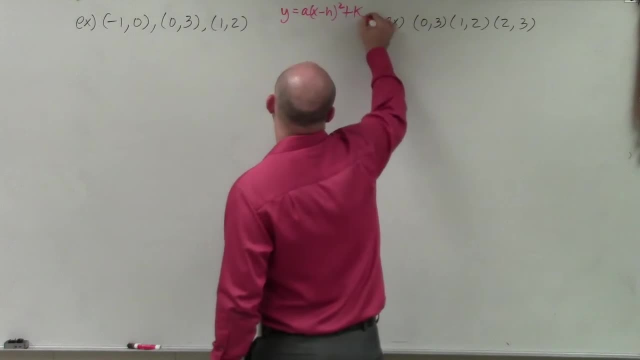 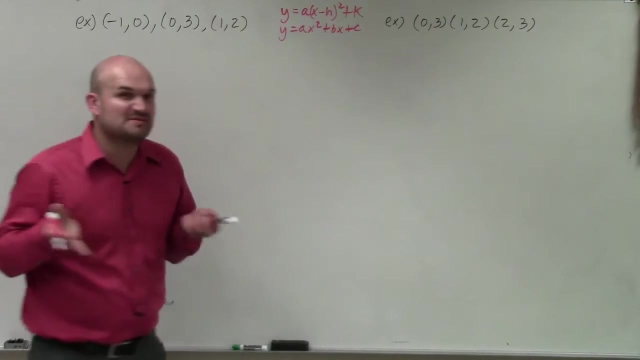 using either vertex form or we were using quadratic form. y equals ax squared plus bx plus c. Now, vertex form was very helpful when we knew the vertex. Unfortunately, here all we know is three points that the graph goes through, So we don't even know the vertex. 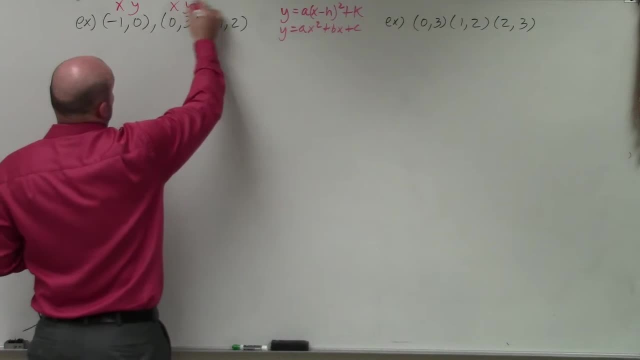 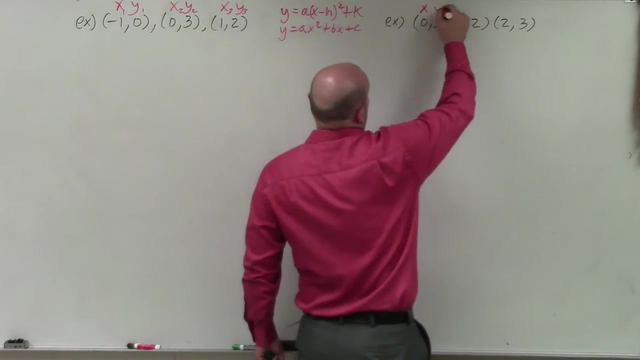 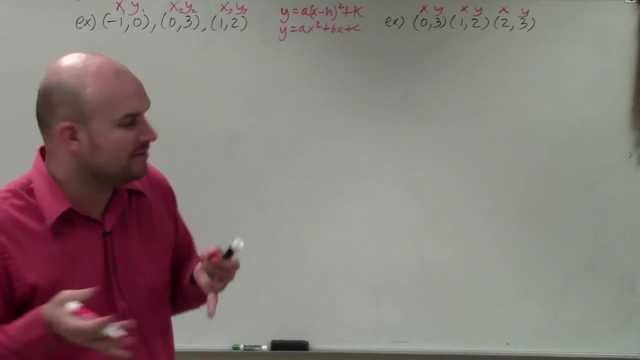 All we have is three points. We have xy, xy and xy. You could label them with subscripts if you like. OK, But you don't have to. Well, anyways, vertex form is going to be kind of difficult for us to be able to write the equation of a line because we only have x and y And. 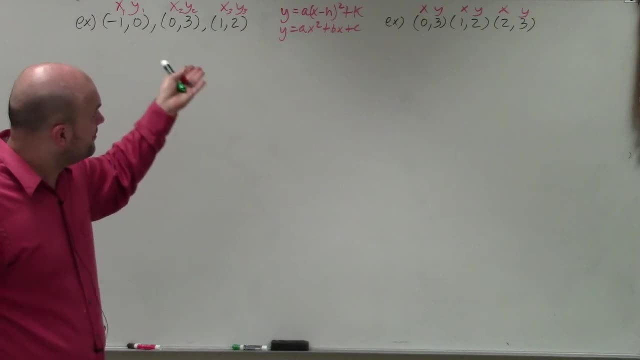 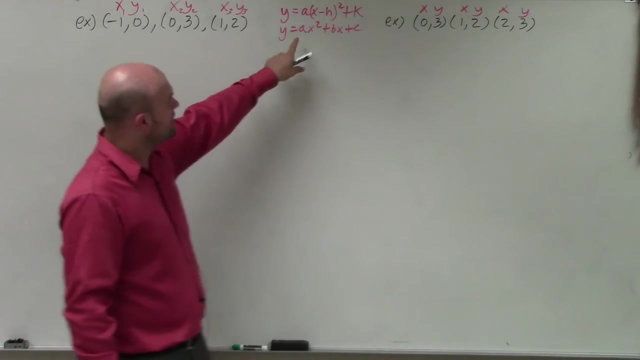 then we still have to go ahead and figure out h and k. However, what we could also do is go ahead and take a look at this and using standard form, Where, in standard form, if you see that we have three points, we also have three variables. 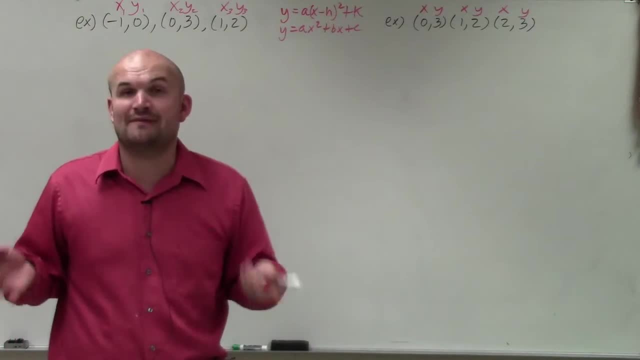 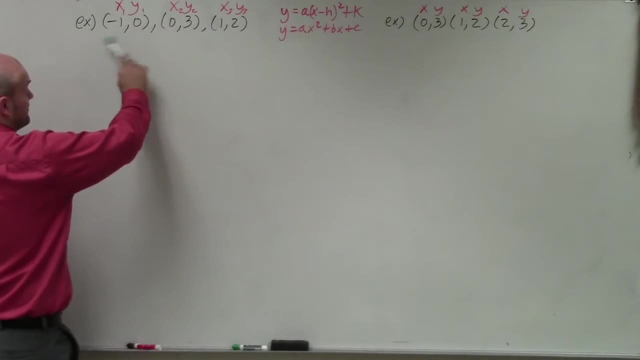 a, b and c, that we do not know, And if we have three variables, therefore, we have to create three equations. Well, that's possible to create three equations. It's possible to create three equations because we have three points And we can plug in these x and y's. 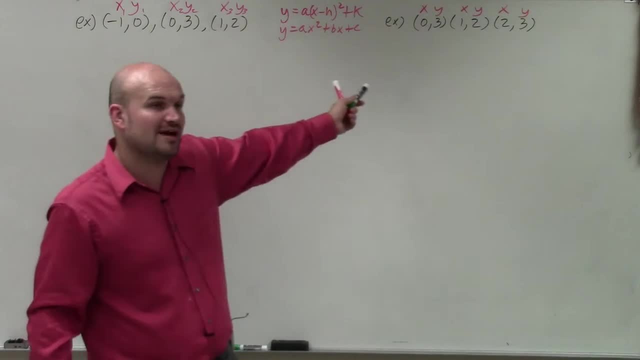 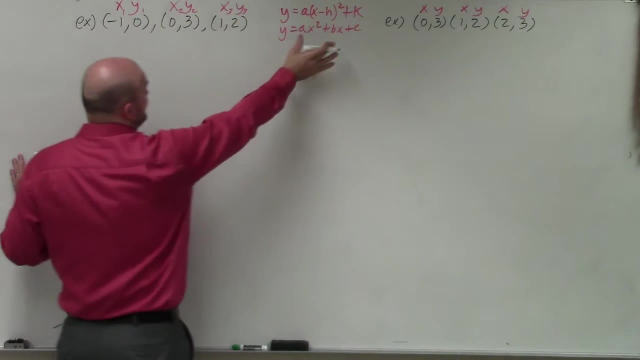 into each one of these into the standard form equation, to produce three equations. And let me go in and explain. Let me show you an example. So basically, what I'm going to do is I'm going to plug x and y into this equation for each of these three points. So my first equation here is: 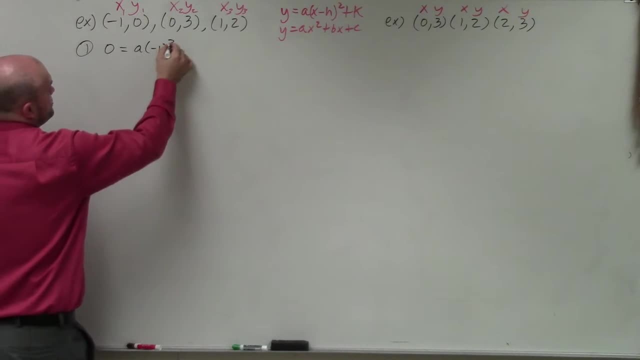 going to be: 0 equals a times negative 1 squared plus b times negative 1 plus c. Then equation number two is going to be: 3 is equal to a times 0 squared plus b times 0 plus c. Equation three: plug in for y. plug in for x. 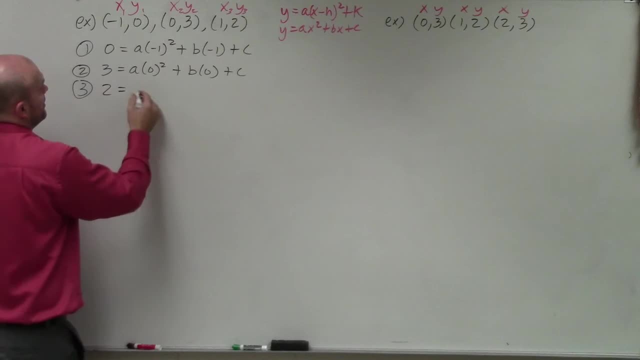 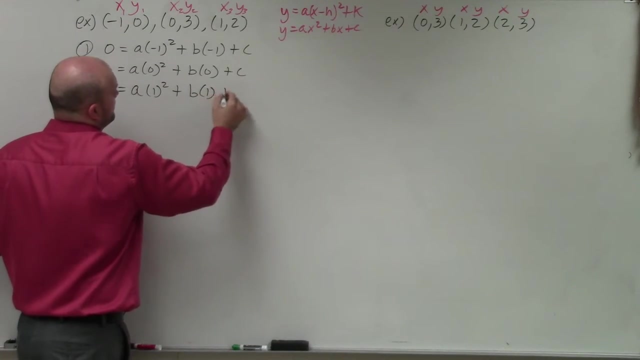 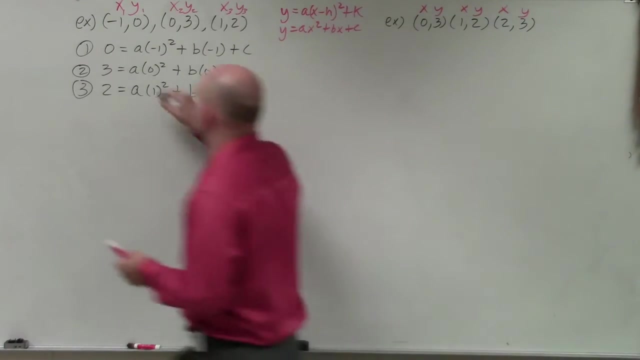 2 equals a times 1 squared plus b times 1 plus c. So now, when I go ahead and simplify this, there's a couple important things that really stand out. First of all, we know that since x is 0 over here, we know that the value of c is going to be equal to 3.. Over here, 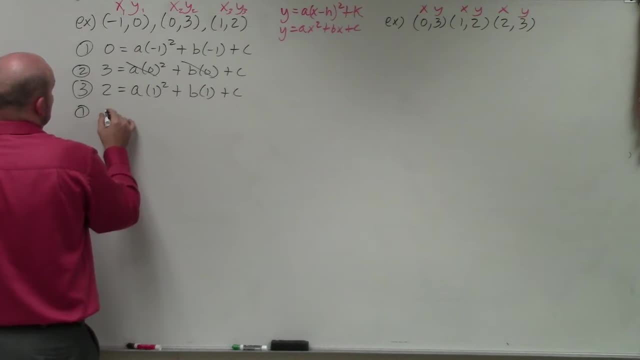 basically I have this equation. Let's go back and rewrite them in the simplified form. So here I have 0 equals negative 1 squared plus b times 0, squared plus b times 1 plus c. So here I have 0 equals negative 1 squared plus b times 1 plus c. So now, when I go ahead and 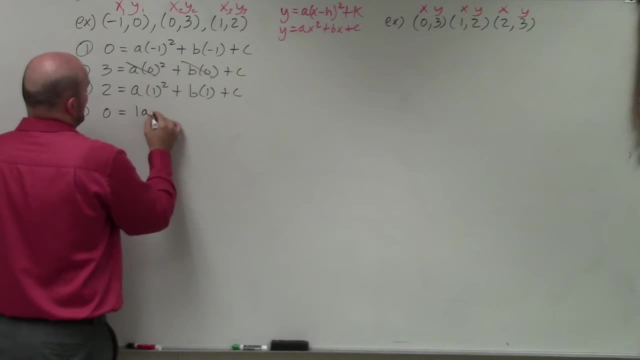 modify this equation. let's say that 1 squared is negative, 1 squared plus 1 times c. So look what this equals. So I have negative, 1 squared is 1.. So that's just going to be 1 times a plus minus b, because negative 1 times positive b is going to be a negative. 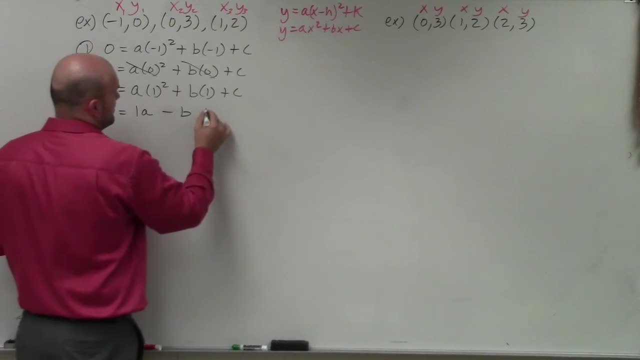 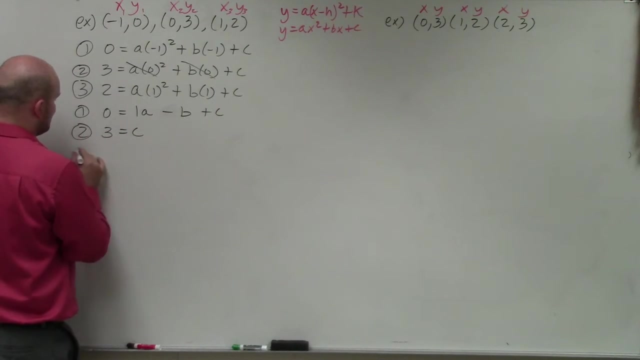 b. So instead of saying plus negative, we'll just keep that as a negative b and then plus c. Equation two: as we mentioned, 3 equals c And equation three: in this case we're going to have 0 equals 1a plus b. 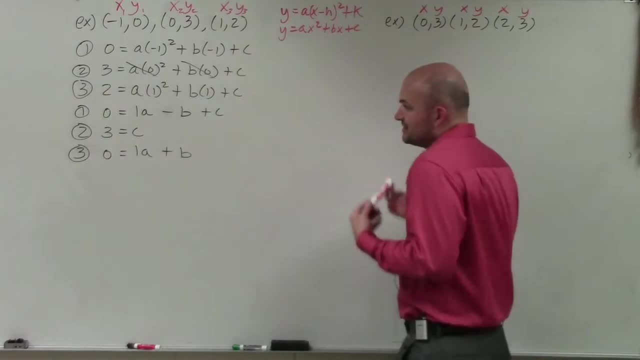 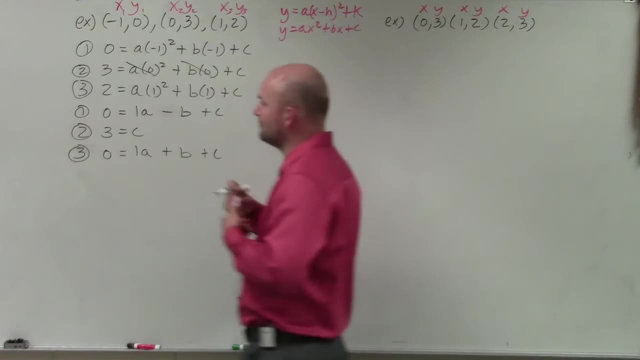 EQUATION FOUR. EQUATION FIVE: you can see that we have three equations, but the nice thing is we now know oops plus c. We now know what the value of c is. So what I'm going to do is I'm going to replace. 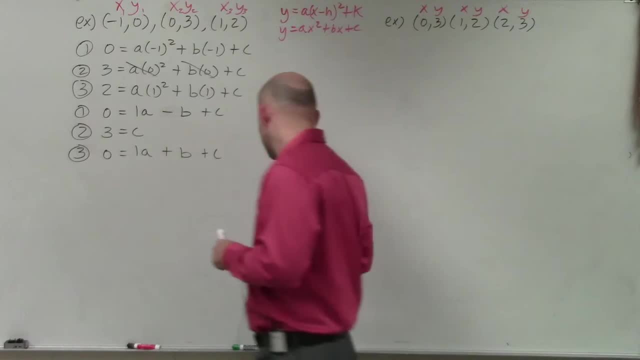 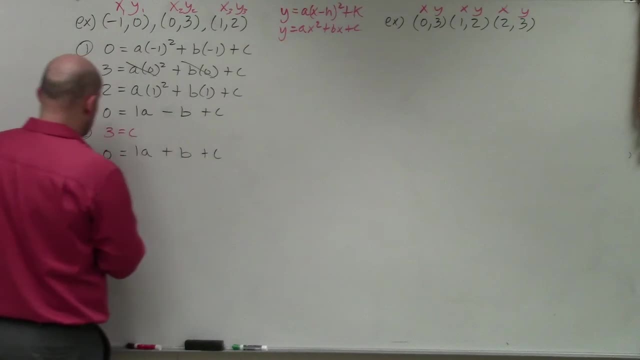 the value of c here and here with the value 3.. So actually I'll write this as 3 equals c. Then what I'm simply going to do is go back to my first two equations and I'll have 0 equals a minus b plus 3, because that's what the value of c is- and then 0 equals. 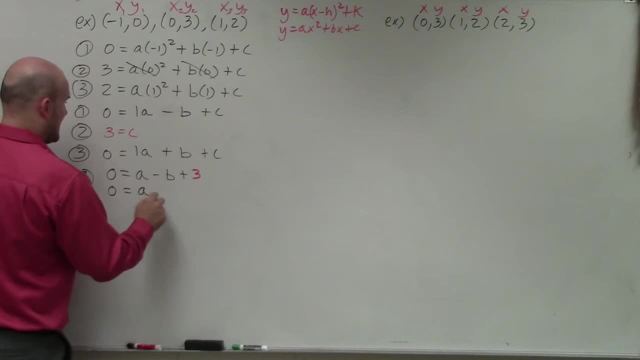 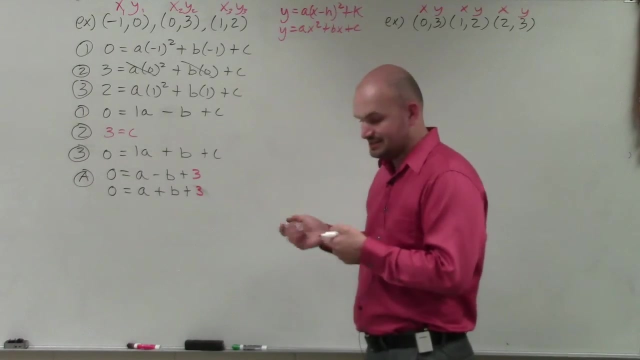 a plus b plus 3.. Okay, plus 3.. Now, if I was going to solve a system that would be quite simple, I would have to do the following: The main important thing that we want to do is make sure we get the variables on the same. 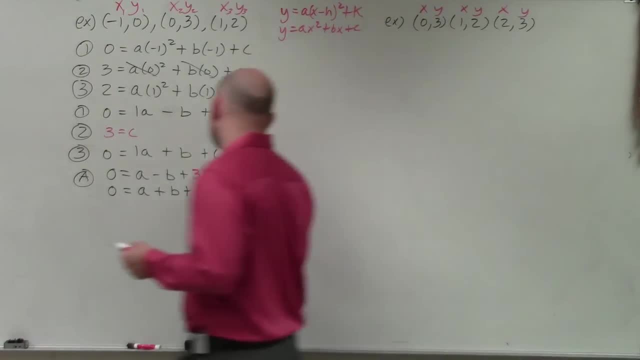 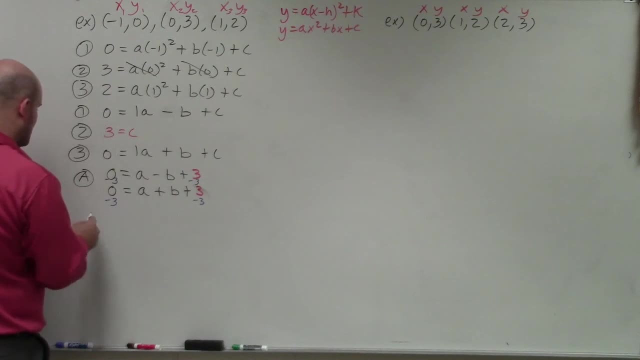 side. So what I'm going to do in this case next is I'm going to subtract the 3 on both sides for both equations. Therefore, I'm going to attain now a new system of equations, which I'll call b, which is negative: 3 equals a minus b and negative 3 equals a plus b. Well, 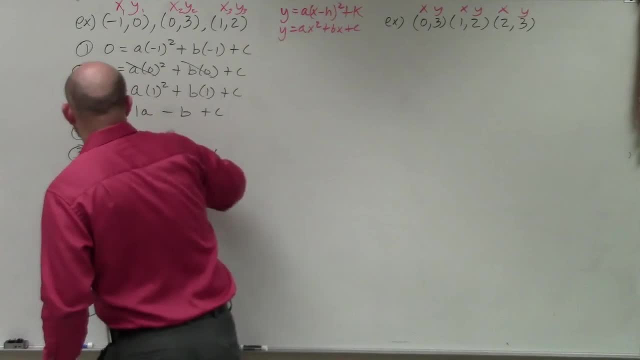 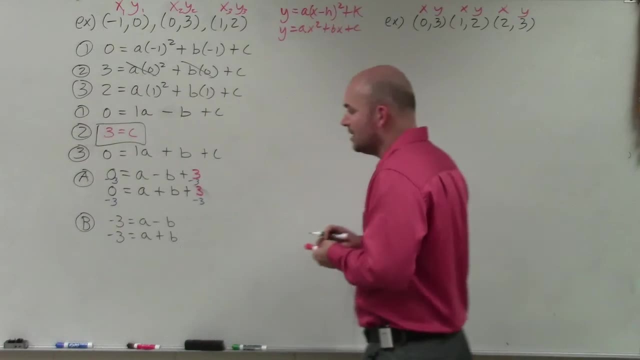 if I want to solve for the values of a- b, because I already know what the value of c is. So if I want to find the values for a and b, I can solve this using a system of two equations, by using substitution. I'm sorry. 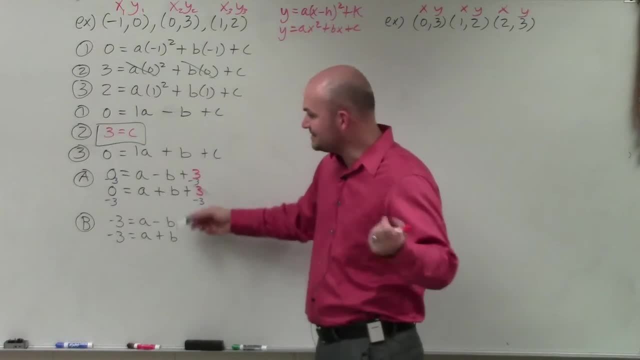 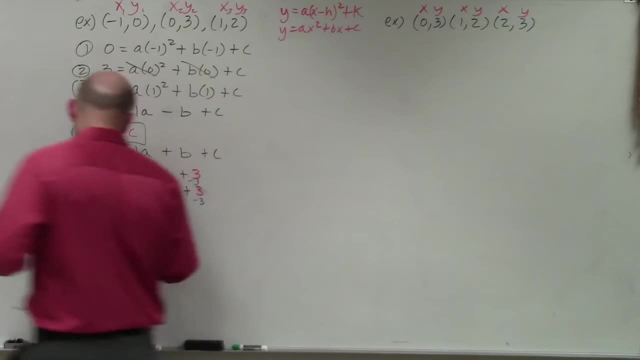 not substitution. You could use substitution, but since I have everything aligned and I see that a or b both have a 1, but 1's negative, 1's positive, I can simply solve this by adding the two expressions out and I'll eliminate the variable b. So negative, 3 plus negative. 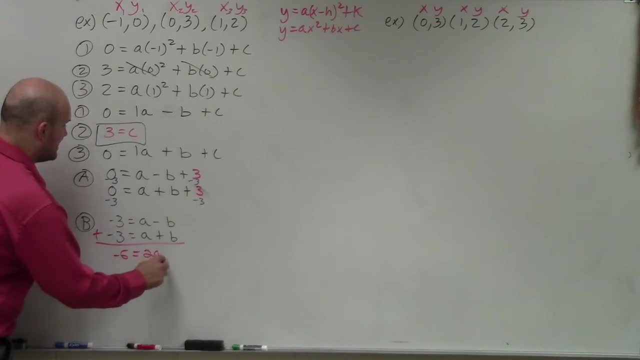 3 is going to be a. negative 6 equals 2a, and negative b plus positive b is going to be a 0b. Then to solve for a, I'll divide by 2,, divide by 2, and negative 3 equals a. So I know c is equal to 3,, a is. 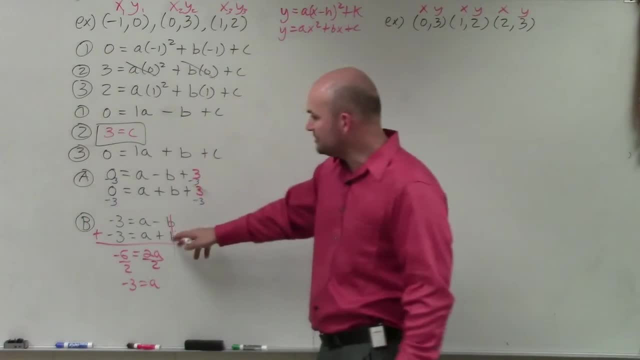 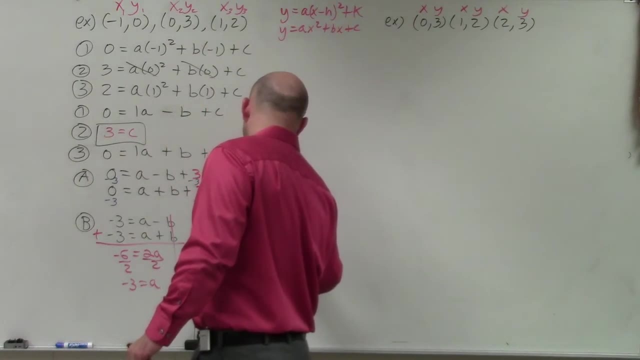 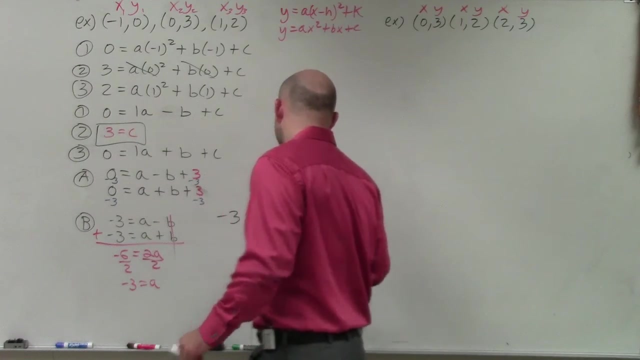 equal to negative 3.. Now to go back and find b, I can simply just plug the value of a into one of these equations, So I'll just do: negative 3 equals negative a. oops, not negative a. negative 3 plus b. Now I'll simply go ahead and solve for b, So I'll just add a 3 to both. 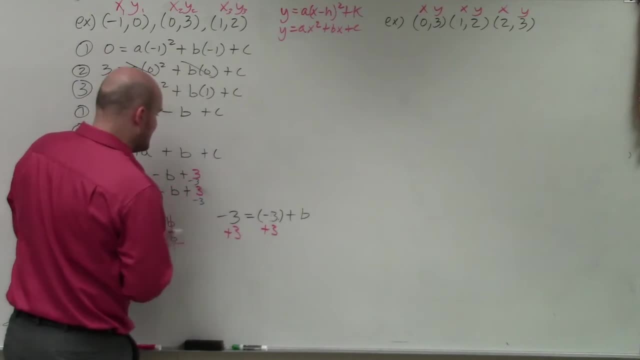 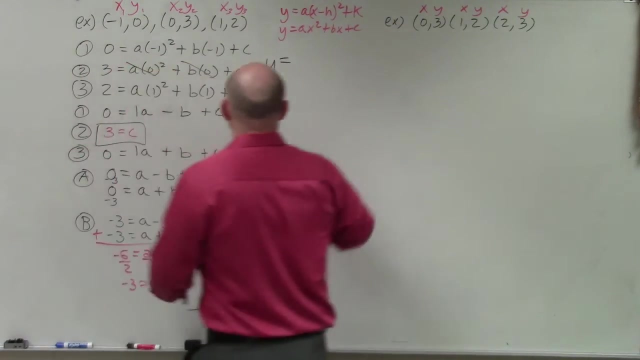 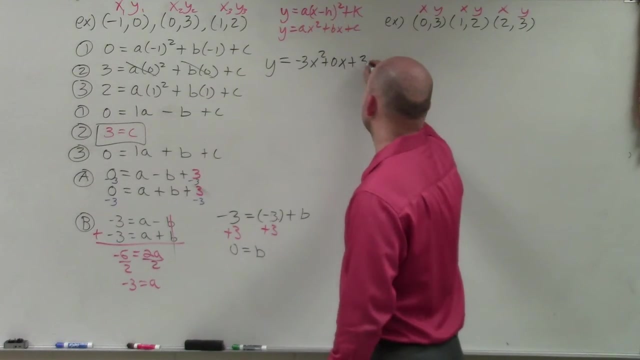 sides And what I get is 0 is equal to b. So writing the equation now in standard form: I know a is negative 3,, I know b is going to be 0, and c is going to be 3.. Well, obviously, 0. 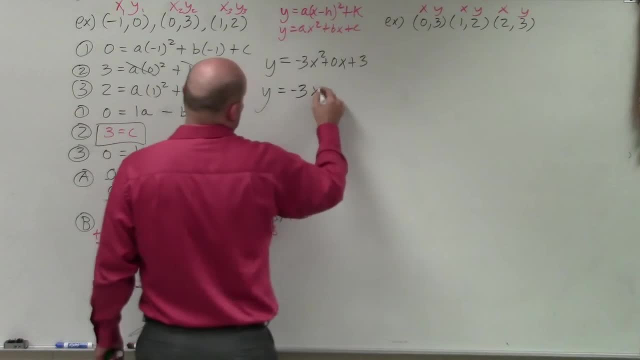 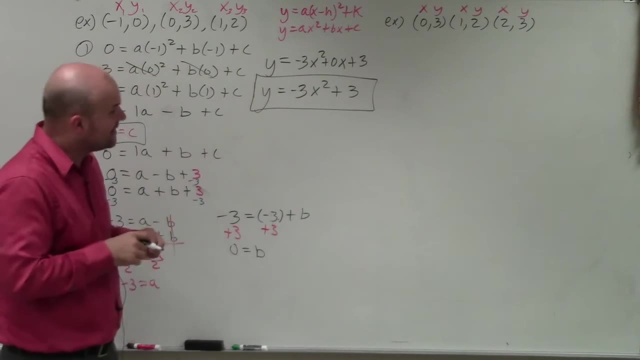 times x is just going to be 0, so my final equation is going to be a negative 3x squared plus 3.. Ta-da, Okay. so hopefully now you kind of got a little bit of an idea of what to do for that one. 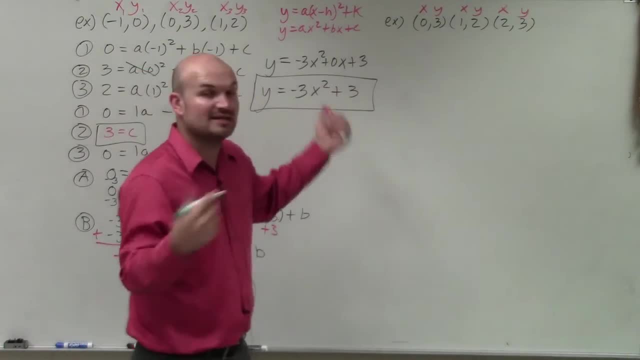 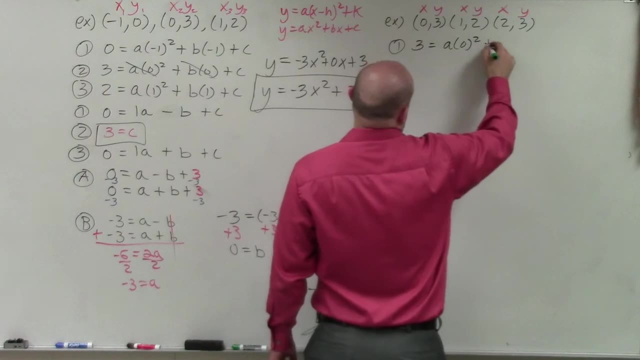 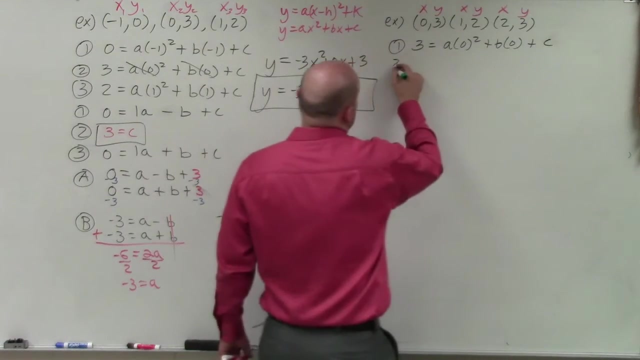 We're just going to do the exact same thing. We have again our xy's. We're going to set up our 3 equation. So equation number 1 is going to be: 3 equals a times 0 squared plus b times 0 plus 3 plus c. Equation number 2 is going to be 2 equals a times 1 squared. 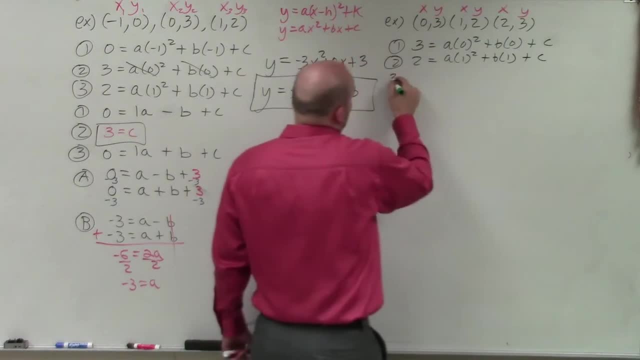 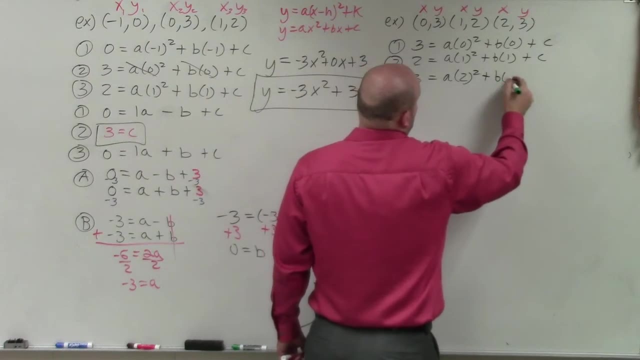 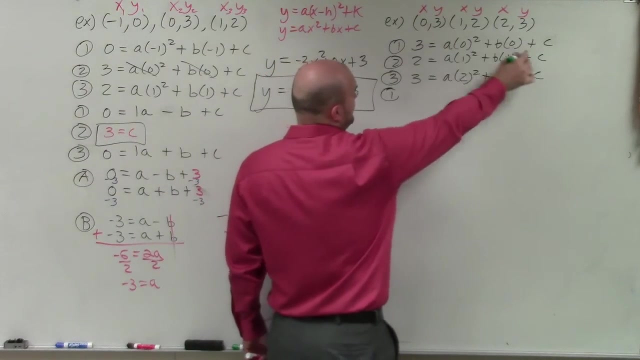 plus b times 1 plus c. And equation number 3 is going to be: 3 equals a times 1 squared plus b times 2 squared plus b times 2 plus c. Okay, Now let's go ahead and simplify each of these equations again. You can see here those that's just going to my zeros. 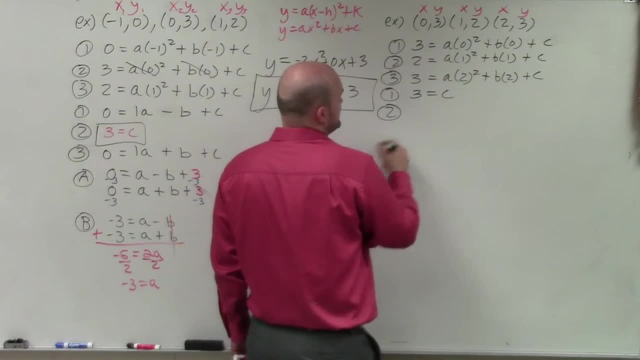 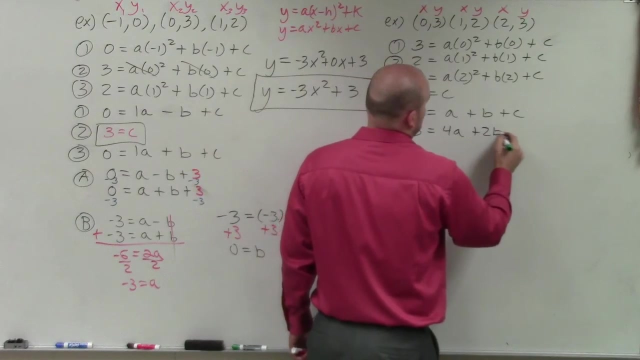 are going to cancel out. so I have: 3 is equal to c. Equation number 2, I can simplify to: 2 equals that's going to be a plus b plus c. And equation number 3 is going to simplify here to: 3 equals 4a plus 2b plus 2c. 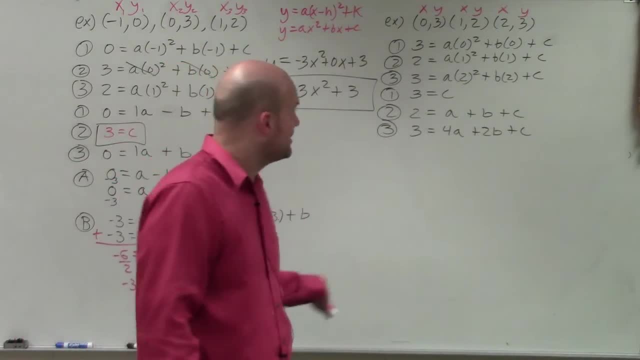 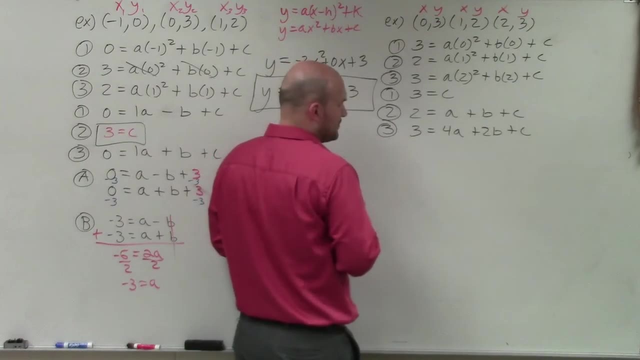 Okay, So now, basically, what I'm simply going to do is, again, I can now evaluate for my value, for my value c, which is equal to 3.. And when I plug in c, when I plug 3 in, for 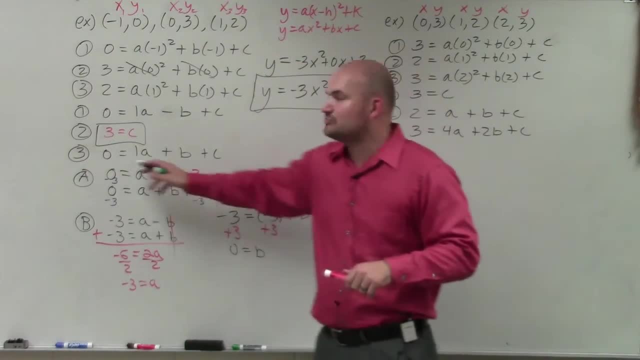 c again, I'm going to have to do the same thing I did over here and then subtract the 3 on both sides. When I go ahead and do that, if I plug in 3,, subtract 3, I have a new systems. 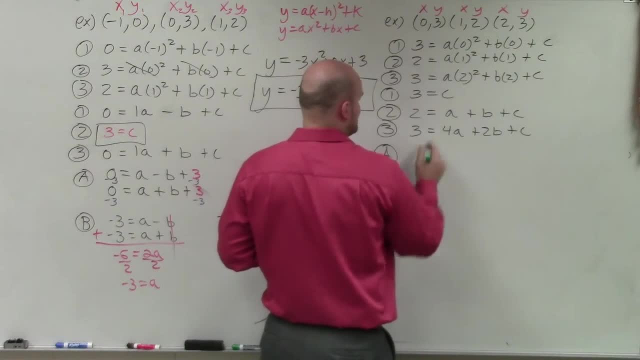 of equations which is going to be: if I have 3 minus 3, it's going to be negative. 1 equals a plus b. And then, over here, if I have 3, subtract 3, I'm going to have 0 equals 4a plus. 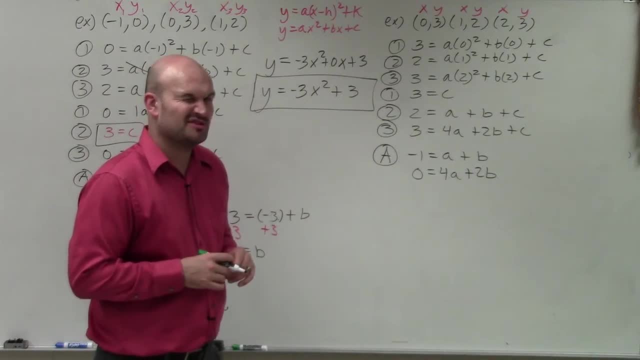 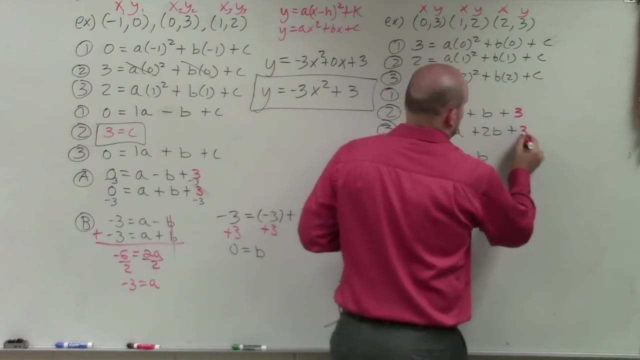 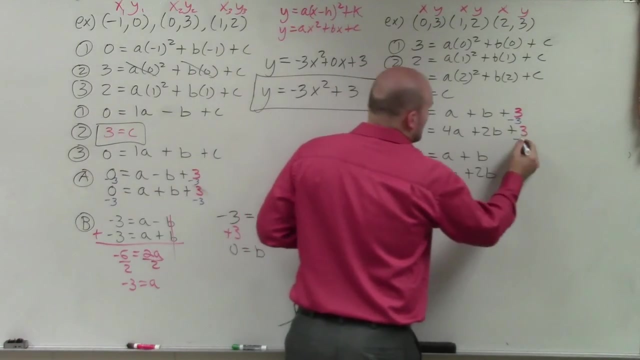 2b. You want me to show you work? Yeah, let's go and show you work real quick. Let's replace this c's with 3.. Then what I simply did was I just subtracted the 3 on both sides. That goes to 0.. Now I'm just. 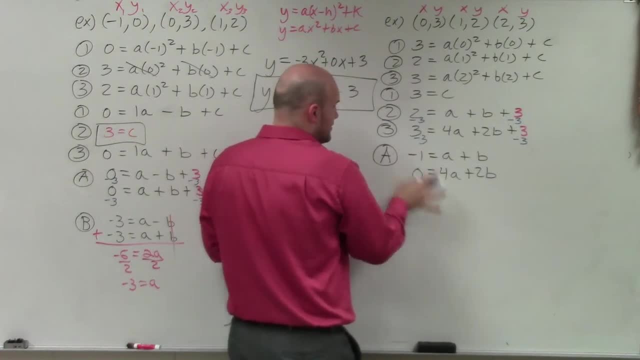 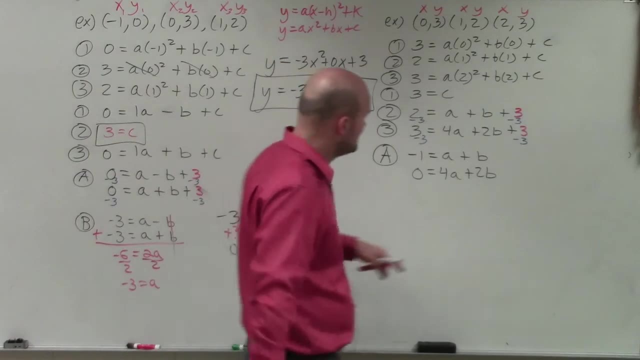 left with the black over here. 2 minus 3 is negative, Negative 1.. 3 minus 3 is 0.. So now I have a system of equations, And to solve the system of equations again I could either use substitution or elimination. Well, you could do substitution easily. That wouldn't. 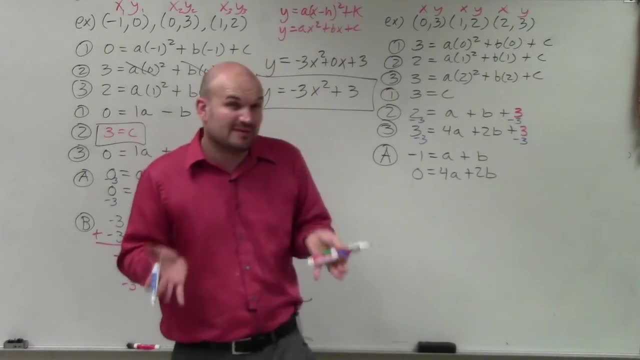 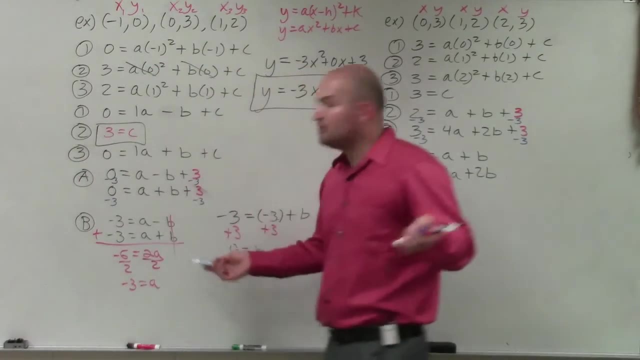 be a problem, But I think using elimination would be the easiest. The main important thing: we just need to identify which variable do we want to eliminate. Do we want to eliminate the a or the b? Well, this one, we eliminated the b first. So let's go and eliminate the. 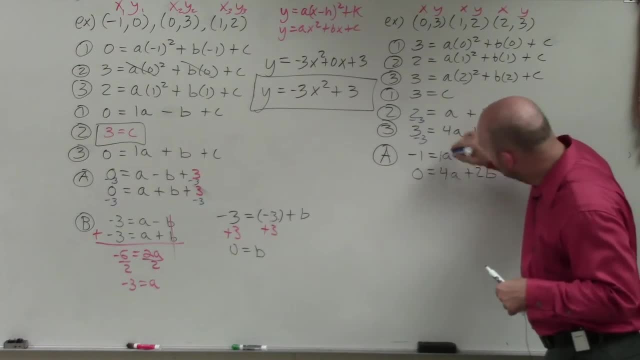 a first. Now to eliminate the a. you see that here I have a 1 as my coefficient And here I have a 4. To use elimination: basically, we're going to be adding them, So we've got to have the. 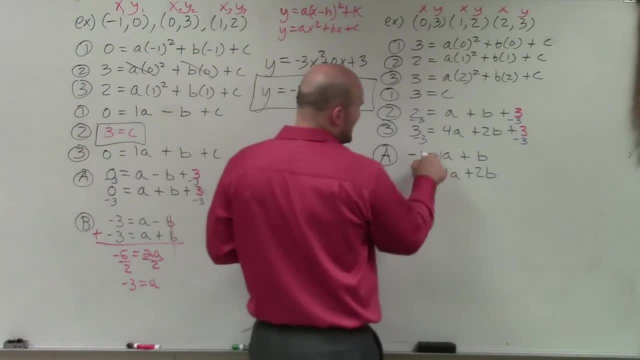 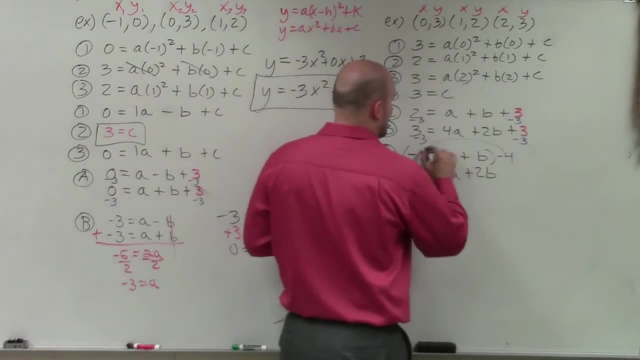 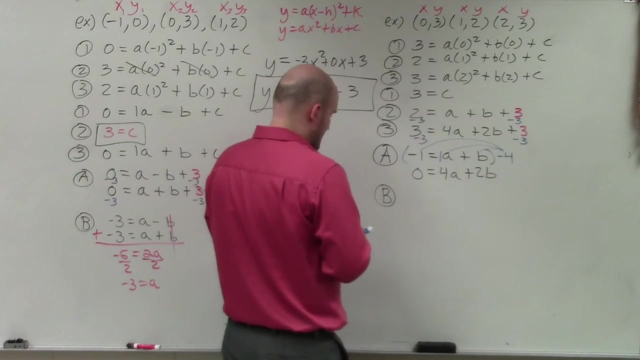 same coefficient, 1 positive and 1 negative. So to obtain the same coefficient for a, I need to multiply the top equation by negative 4.. And remember you have to multiply every single term times negative 4.. So when doing that, I obtain a new system of equations which I'll call b And I now 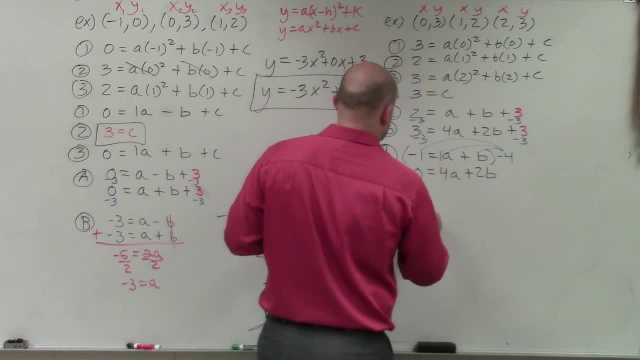 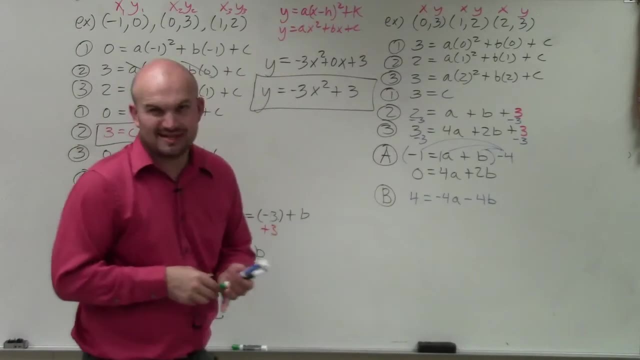 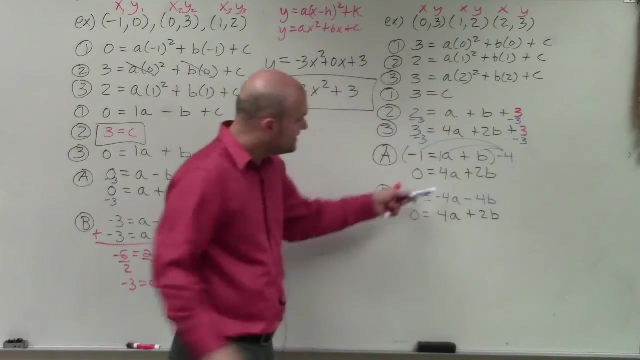 get 4 equals negative, 4a minus 4b, b, because it's really plus a negative 4b, and then below I'll have 0 equals positive, 4a plus 2b. Now you can see that a has the same coefficient: 1 negative 1. 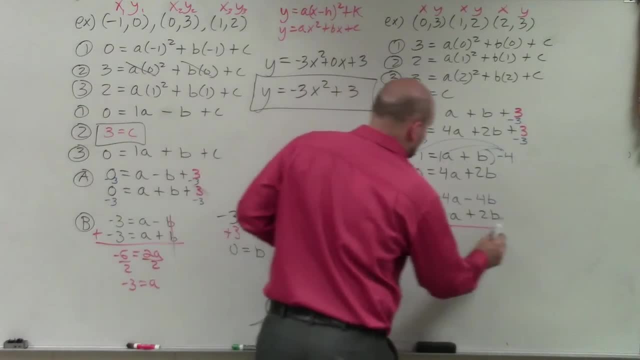 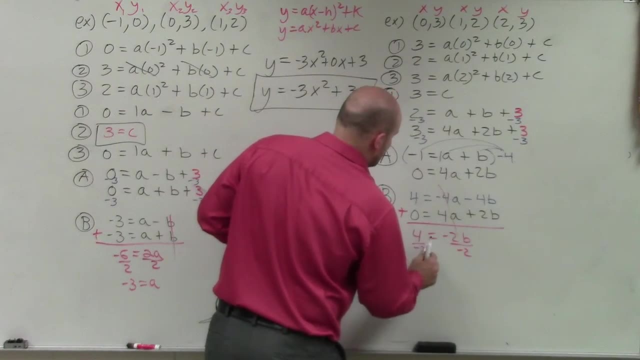 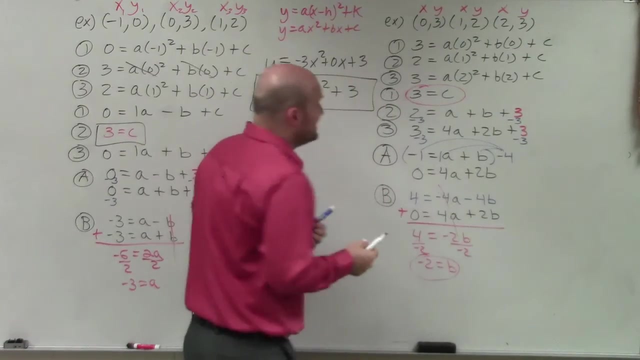 positive, and now I can just add them up and then those are going to divide out. I have 4 equals negative, 2b divided by negative, 2. divided by negative 2, negative 2 equals b. So I know what the value of c is. I know the value of b Now. 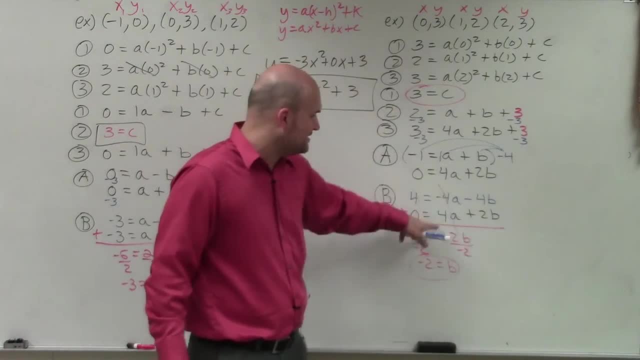 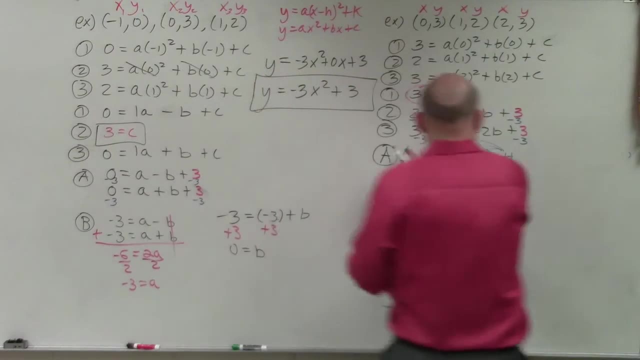 all I simply need to do is again plug this value b into one of these two or one of these two equations. You could plug them into these two, but these are the more simplified Plug in with these two to find the value b. So I'm going to plug in. 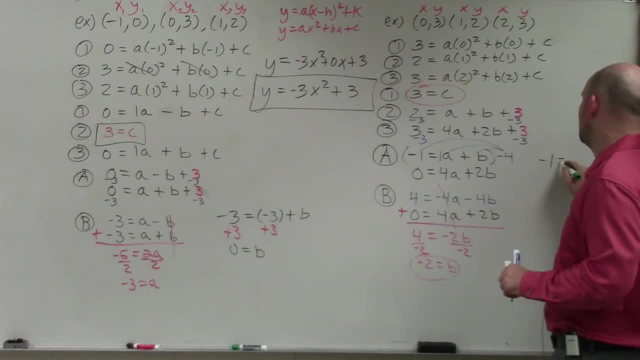 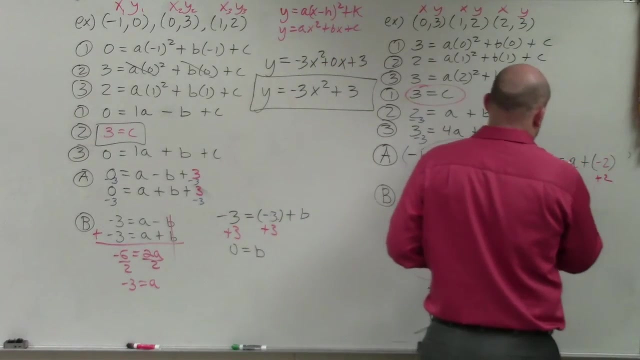 the top equation before I entered in negative 1.. So I have: negative 1 equals now negative 2 or a plus negative 2.. So now to solve for a, all I simply need to do is add a 2 to both sides and what I get. 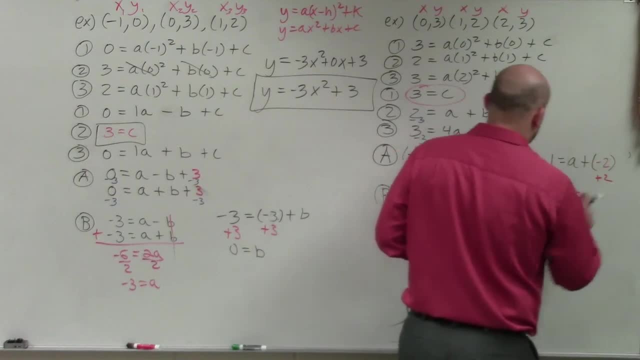 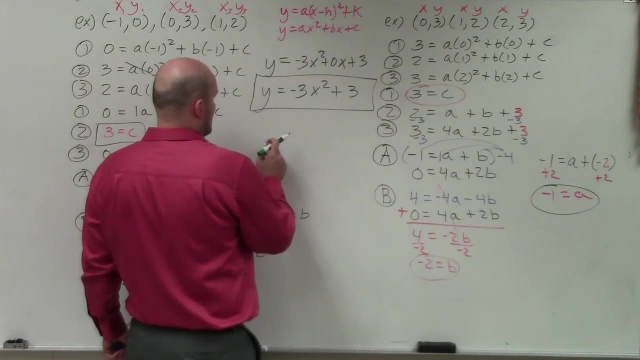 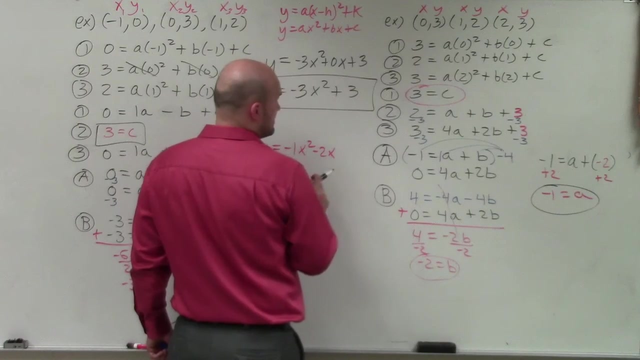 is is going to be negative. 1 equals a. So now I know what a, b, c. So to write my equation, it's simply going to be: y equals negative, 1 x squared minus 2x plus 3.. And then obviously I don't need to write that 1 there.